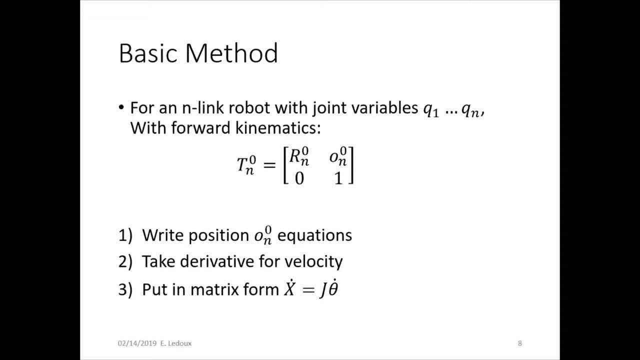 These are the equations that get the numbers in the position spot of the homogeneous transformation. So then we take the derivative of those equations to get velocity and put it in matrix form: x dot equals j theta dot, where x dot is end-effector velocity and theta dot is joint speeds. 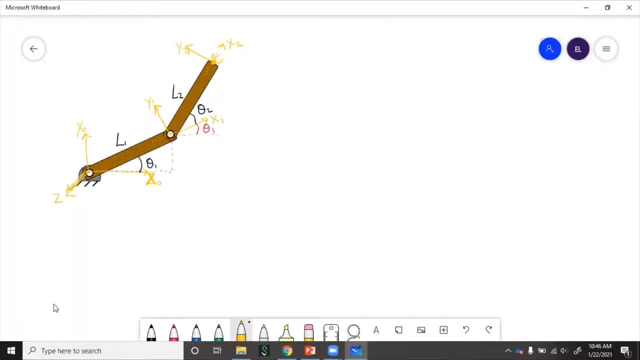 So let's do an example of this Here. we'll do an example using the two-link robot and find the Jacobian of this. Step one is find the forward kinematics. Step two is take the derivative and get velocity. Step three is put it in matrix form. 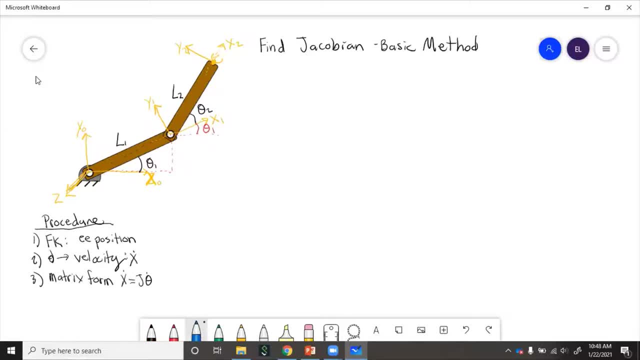 So we'll start with step one, getting the x, y, z positions of the end-effector. So x, y, z, z equal to небольшide 정도, be i out here- or y equal to zero. So this is going to be x-position of this. 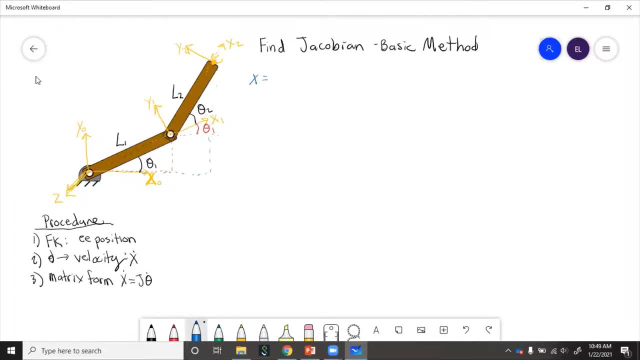 So we'll go all the way out here to the side and then all the way up To get to the end-effector. we have to travel along the link. So first link one And then link two, And it's cosine of theta 1 plus theta 2. 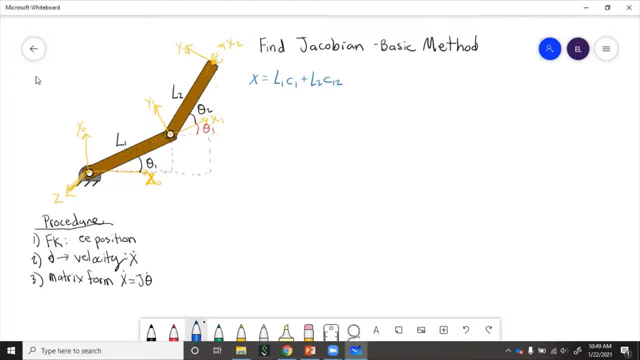 because theta 2 is given with respect to link one to get the angle of link 2.. So now we take the derivative of these and get velocity. Remember to use product rule because cosine of theta1 plus theta2 is going to have theta1. 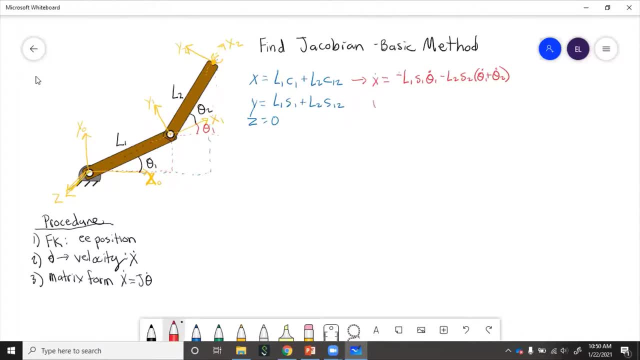 inside of it and theta2 inside of it. Next, we put these in matrix form. So we're going to put these in matrix form. So we're going to put these in matrix form. So we'll have the x? dot matrix, which is really x dot, y dot, z dot.